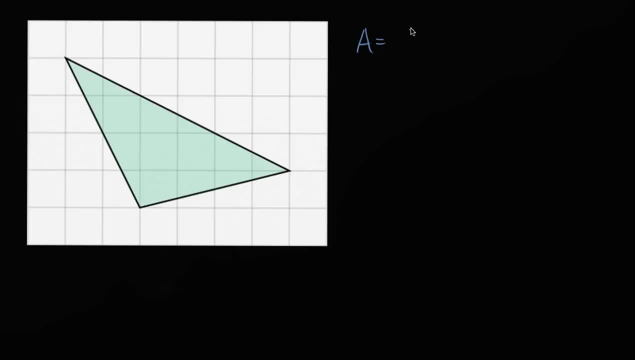 or at least my brain says: well, look, I can figure out the area of a triangle. if I know the base and the height of the triangle, I can just multiply them and then multiply that by 1 half. So, for example, if I have a triangle that looks like this: 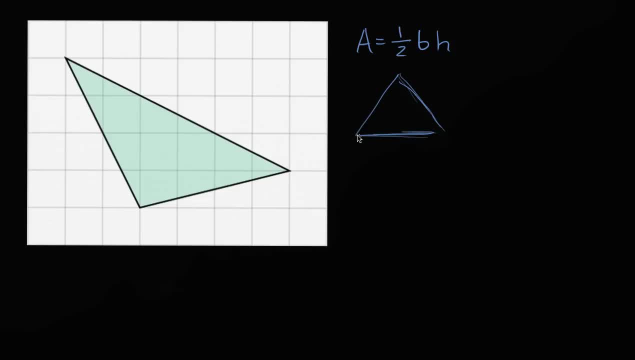 and if this is the base, this is b right over here. The length of this side is b. Let me put the b in magenta And then the height. let me do that in yellow. This is the height. Then I just multiply base times height times 1 half. 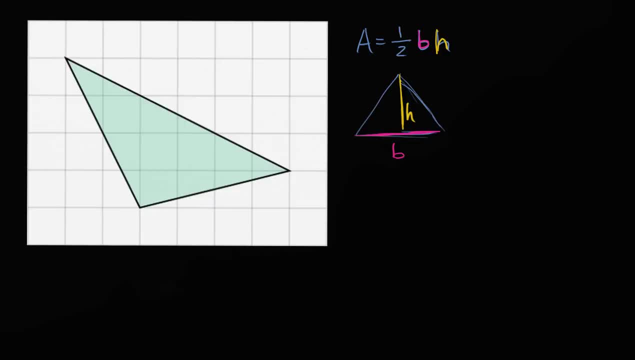 and I'll get the area of this triangle. Or if the triangle looked like this, I could do the same thing Where: if this is the base b, so that is the base b And now the height. I guess you could say this: 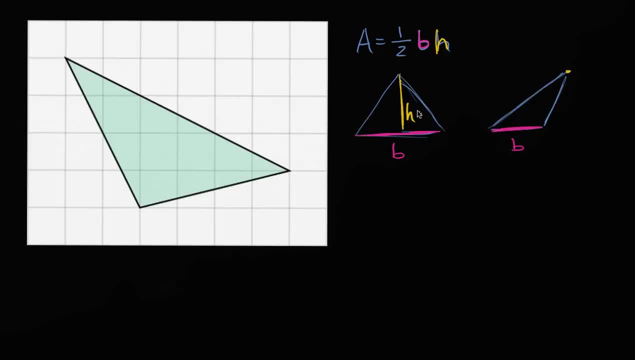 if you were to drop a penny from here. it's sitting outside the triangle so it looks different than this one, But this would still be the height. This would still be the height. right over here You do the same thing: 1 half times base times height. 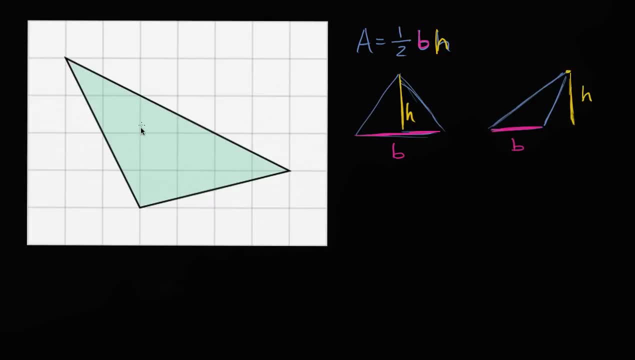 would give you the area of this triangle. So how can we apply that over here? Well, this triangle is on this grid but it's kind of at an angle With this grid. it's hard to pick out the base and the height for this triangle as a whole. 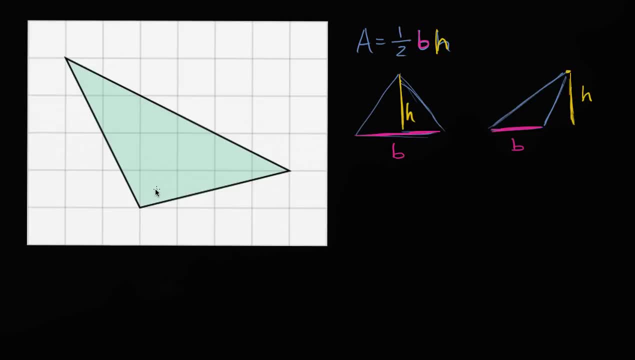 But what we could do- there's actually several ways that we can approach this- is we can break this triangle up into two or more triangles, where we can figure out the base and the height for each of them. So, for example, I can break this one. 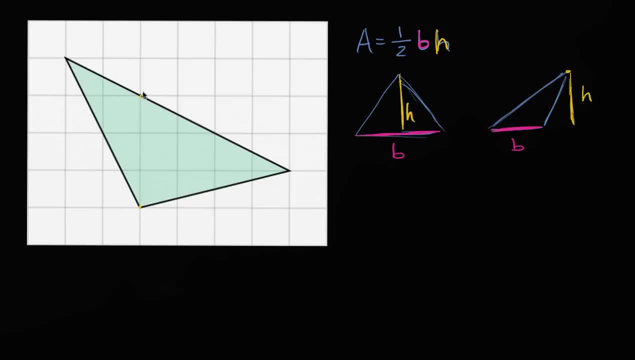 Let's see I could. I'm picking this point and this point because it breaks it up into two triangles where I can figure out the base and the height. Well, what am I talking about? Well, this triangle over here that I am shading in blue, 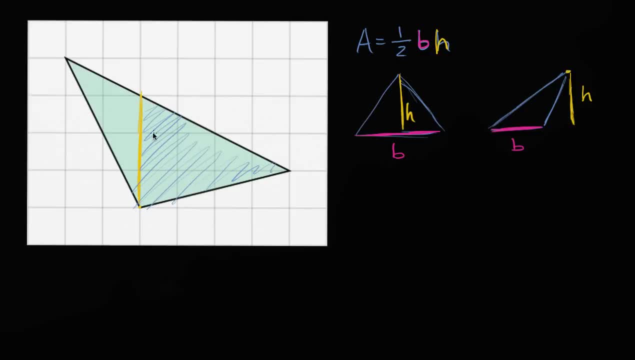 if I, and I've switched the orientation, I've rotated 90 degrees, But if you view this yellow, if you view this yellow as the base of this triangle, you see that the base is 3.. So let me write: the base is equal to 3 units. 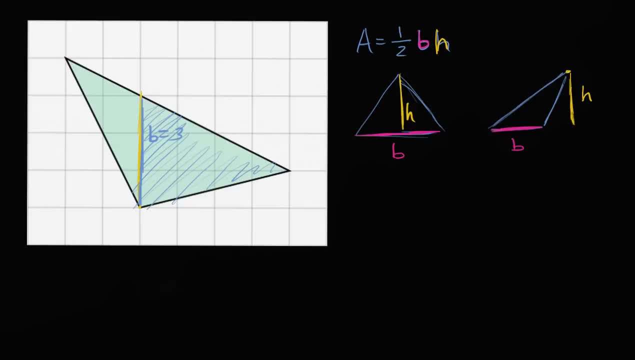 And what's the height here? Well, the height here is going to be, the height here is going to be this distance right over here, Which is 4.. Height is equal to 4.. So the area, the area of that triangle right over there, 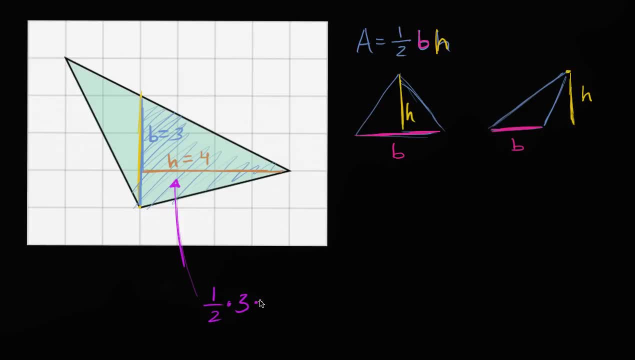 is going to be 1 half times 3 times 4. Which is equal to 6.. So this part right over here, the area is 6.. And now we can do a similar thing with this other triangle, Because, once again, 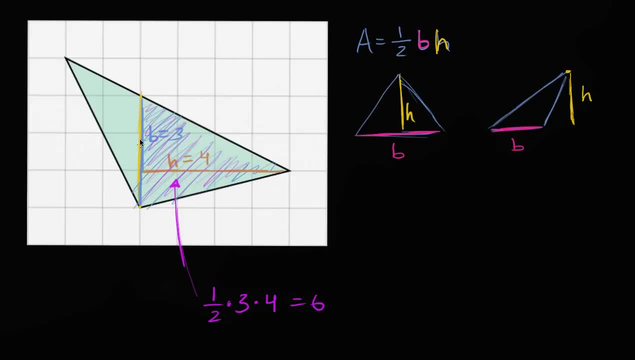 we can view this yellow line, or now I have this yellow and blue line as the base. The base is equal to 3.. So I could write that base is equal to 3.. And once again I've rotated, so now the base is on the side. 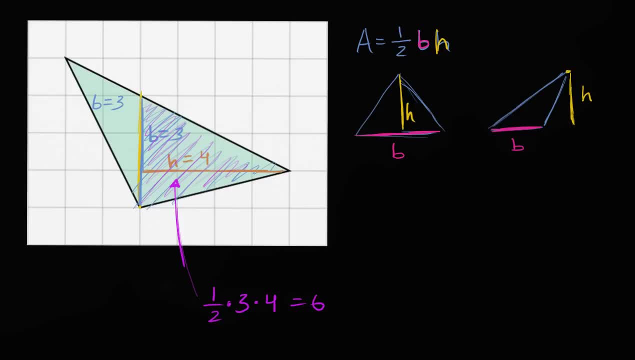 So the base is 3.. And then the height: here the height of this triangle is 2.. If this is the base- remember, if this is the base- here we've just rotated it- then this right over here is the height. 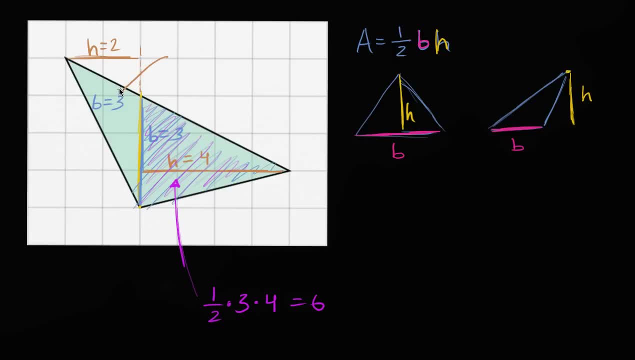 Height would be equal to 2.. So what's the area of this one? The area of this one is going to be 1 half times the base, 3 times the height, which is 2.. 1 half times 2 is 1,. 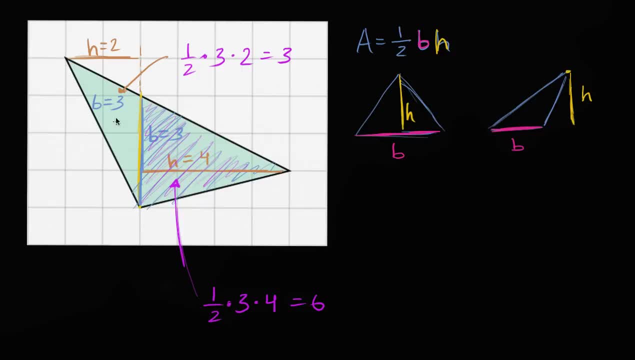 times 3,. this is going to be equal to 3.. So the area of the whole thing is going to be this area of 3, plus this area of 6, is going to be an area of 9.. Area is equal to 9.. 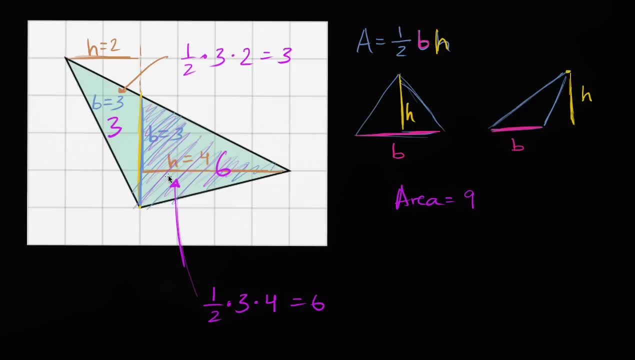 Now, that's one way you could do it is you could break it up into triangles where you could figure out the base and the height Another way- and this is, you can kind of view it as a maybe a trickier way- 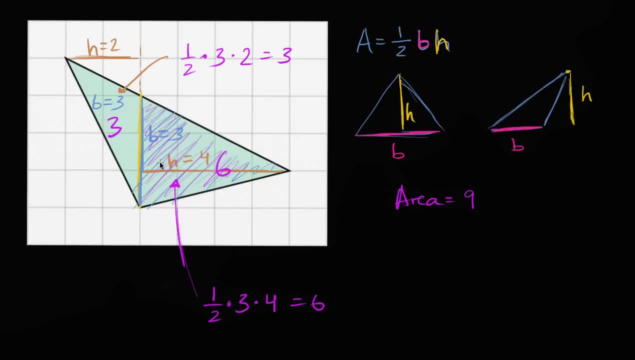 or you kind of have to think a little bit outside of the box or maybe outside of the triangle. to do it this way is to, instead of doing it this way, visualize this triangle, And actually let me clean this up a little bit. 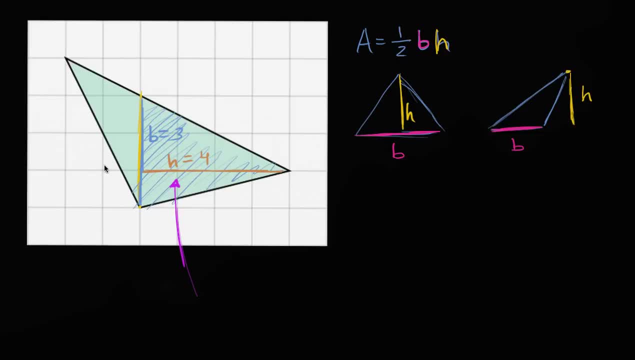 Let me undo all of this work that I just did. Let me undo this to show you the other approach, the other way that we could tackle this. So the other way we could tackle it, and I'm going to clean up the whole thing. 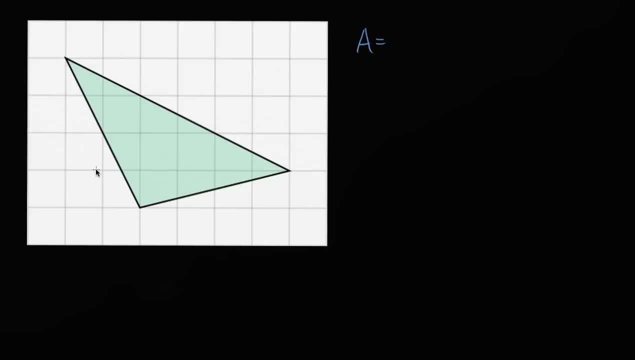 so I get more real estate here. So the other way that we could tackle it is imagine that this triangle is embedded inside of a rectangle. So let me draw the rectangle, Let me draw the broader rectangle, and I think you might see where this is going. 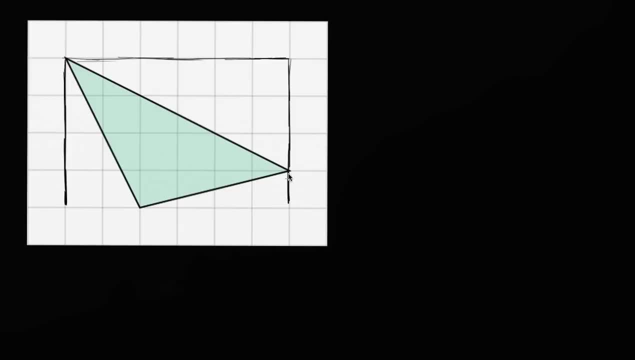 Because as soon as you draw that bigger rectangle, then you see that that rectangle is made up of the triangle that we're trying to find the area of and three other right triangles. We have this right triangle that I'm shading in in yellow. 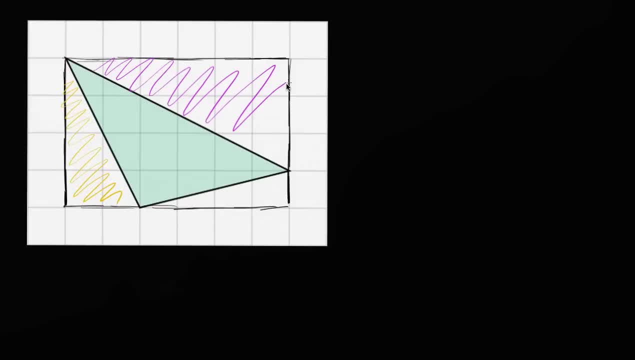 We have this right triangle that I'm shading in in purple, And then we have this right triangle that I am shading in in blue. So if we figure out the area of the entire rectangle- and that's pretty straightforward- the area of the entire rectangle. 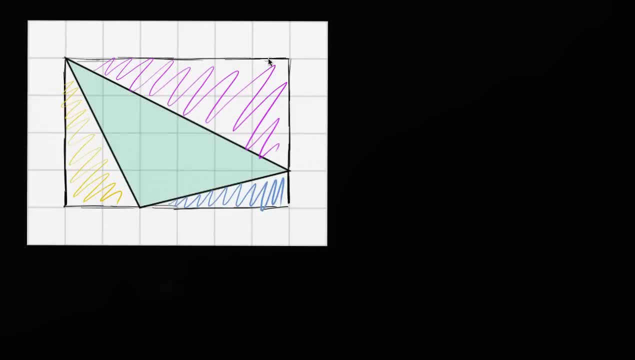 is going to be four times six. those are the dimensions of the rectangle four times six. So the area of the entire rectangle is 24.. And then you subtract out the area of the purple, the blue and the yellow triangles. then you're going to be left with the area. 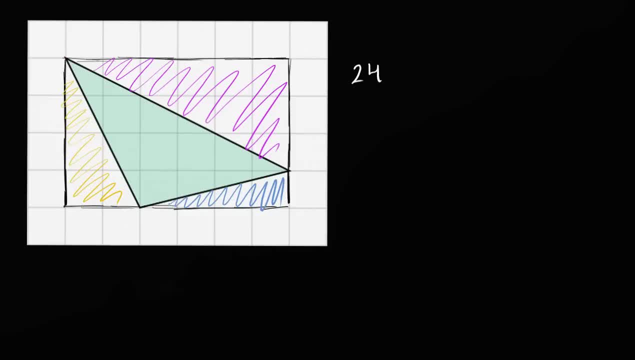 of the green triangle. So let's do that. So what's the area of the purple one? Well, this is going to be- we're going to subtract out, it's going to be one half six its height, right over here. if we view this as its height is six. 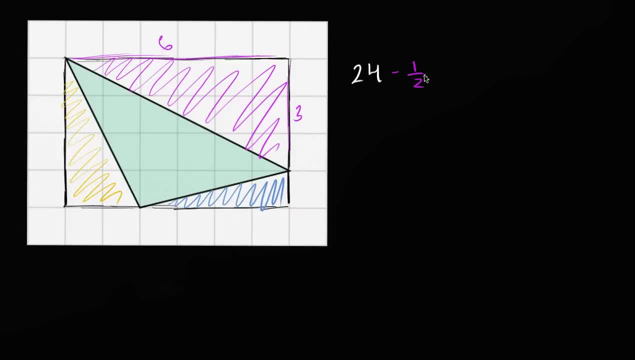 and its base right over here is three. So it's going to be one half times six times three. That's the area of the purple triangle. And then you have the blue one. This is going to be minus one half. let's see, you could say its height is one. 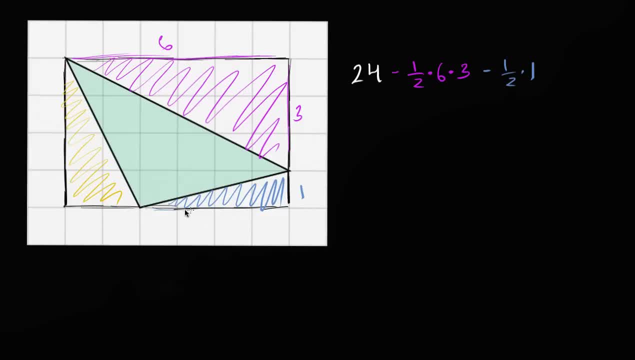 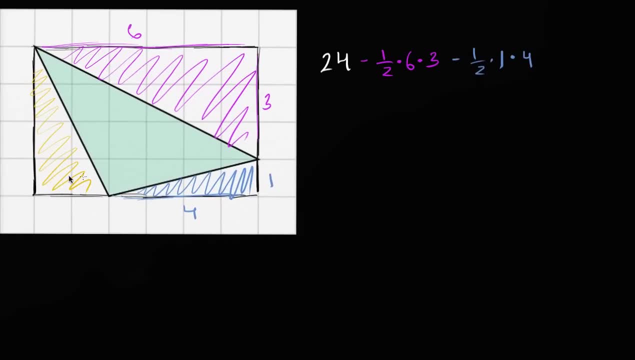 So this is one, And then this base you could say is four. So that's four Times four, And then we want to subtract out the area of the yellow rectangle. So this is minus one half. Let's see we could make this base two. 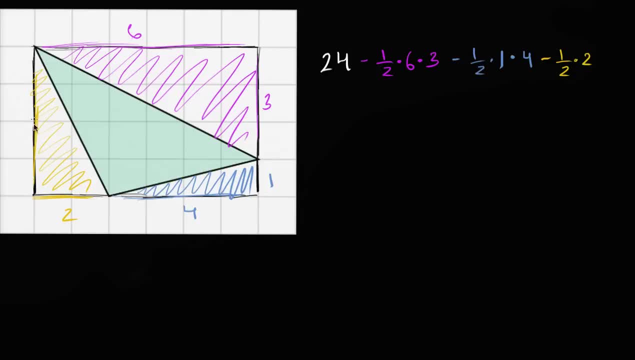 One half times two times, and this height is four, Two times four. So what's this going to be? Well, let's see: One half times six times three, That's three times three, That's going to be nine. One half times one times four. 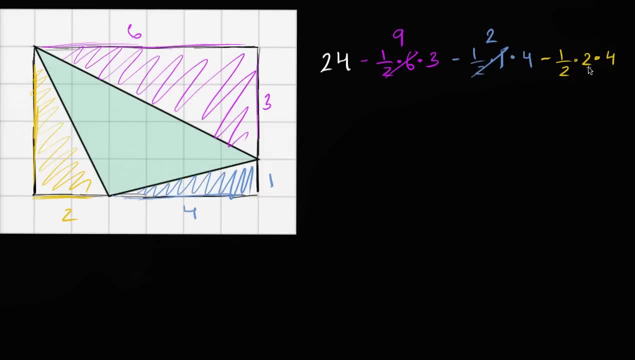 That's going to be two, And then one half times two times four. Well, that's just going to be four, And so we're left with 24 minus nine minus two minus four. So this gets us. let me do the same color.